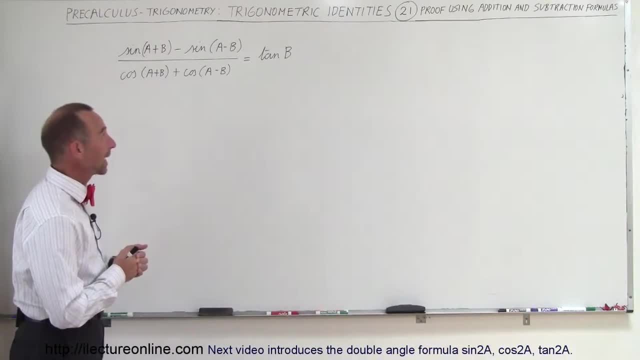 Welcome to our lecture online, and since we know the identities for the sum and the difference of angles, we're going to use that now to prove this particular identity. This is kind of a classic identity. We have the sine of a plus b minus, the sine of a minus b, divided by the cosine of a plus b plus the cosine of a minus b, and that's supposed to be equal to the tangent of b. Doesn't seem likely, but let's see what happens. So first of all let's write this out. So we have the sine of a times the cosine of b. 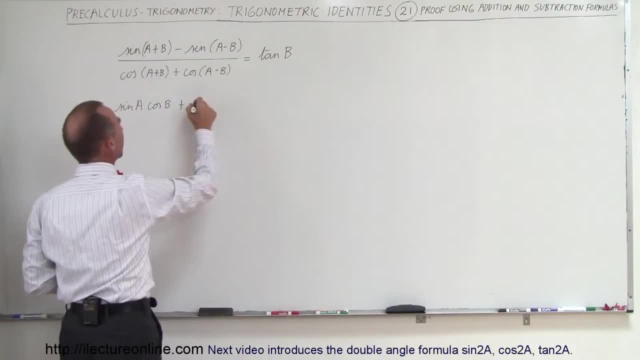 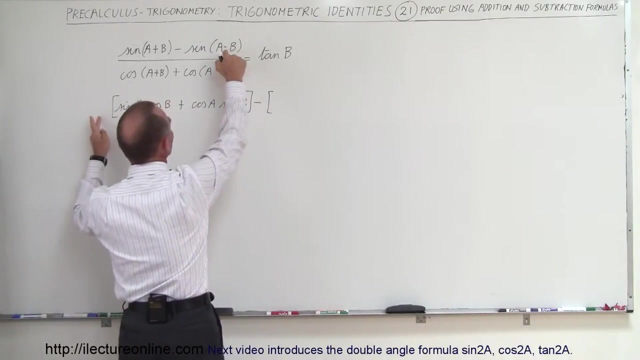 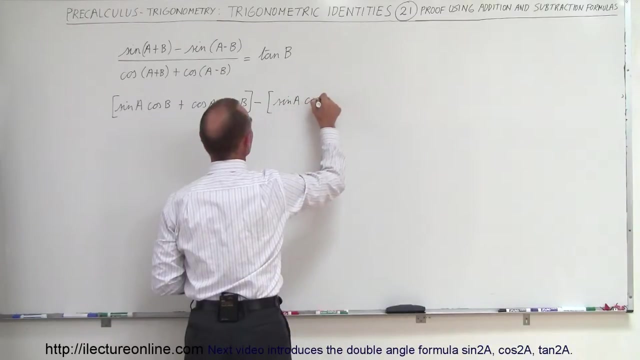 Plus. if this is a plus, we make this a plus the cosine of a times the sine of b. Alright, so this is now represented by that. Let me put brackets around. it makes it easier to see that Minus this right here and it's the same thing as what we had here. but if this is minus, this becomes a minus here. So we have the sine of a cosine of b, and so minus cosine a, sine b. 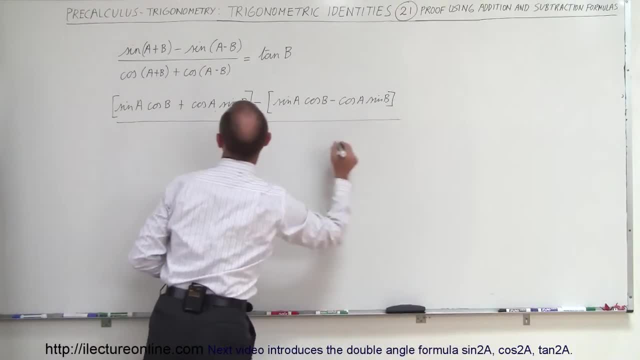 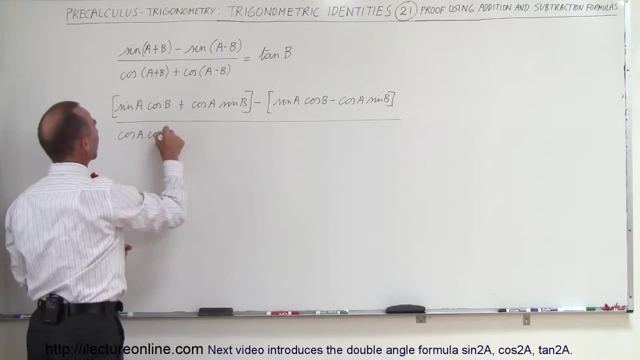 Now we take the whole thing and divide it by. okay, with the cosine it's a little bit different. so see, if you remember, So this would be the cosine of a times the cosine of b, and if this is plus, this becomes minus, and now we get the sine of a times the sine of b. 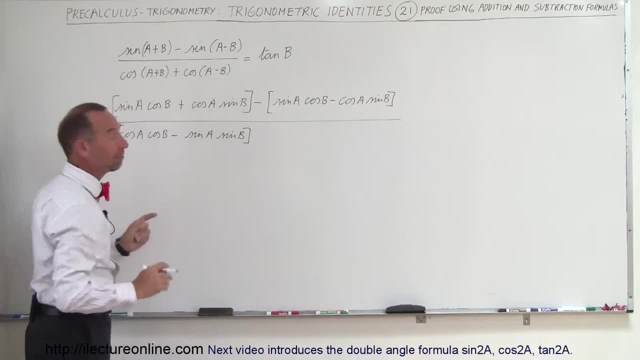 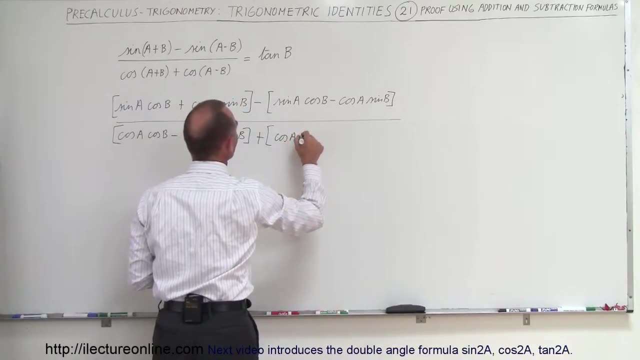 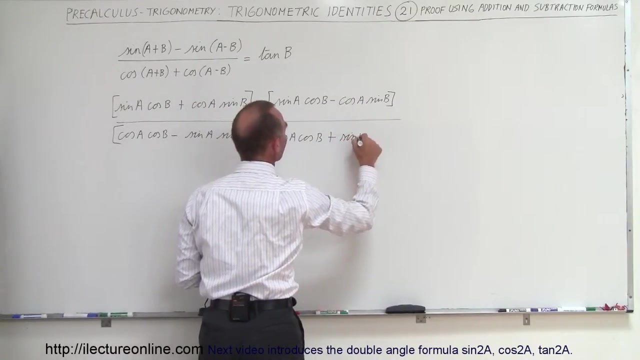 Put brackets around that. so this is now represented by that. and finally, we add to that what this is equivalent to. so this becomes the cosine of a times the cosine of b, And if this is a minus, then this becomes a plus, and this is the sine of a times the sine of b. 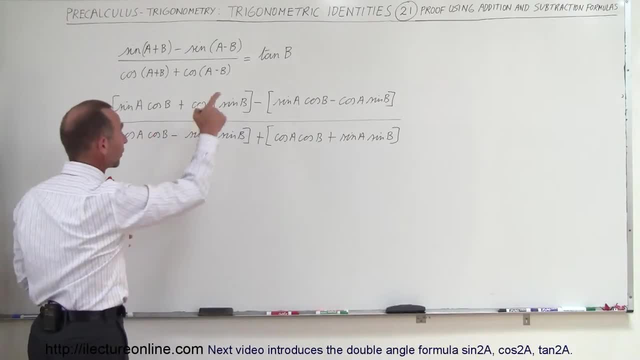 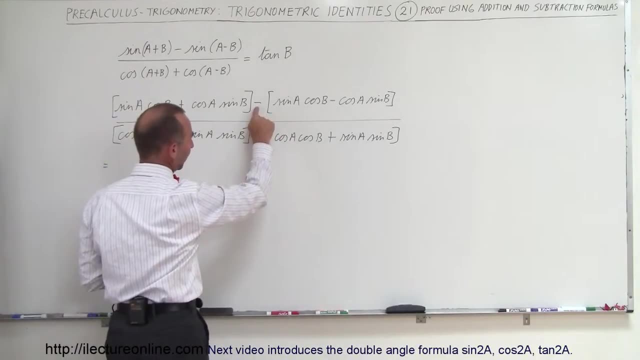 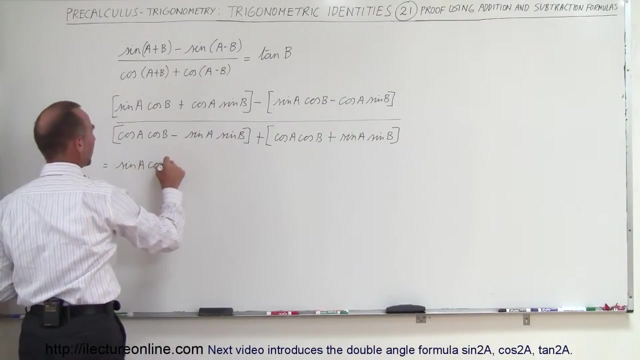 Alright, now let's see if that result completely turns into the tangent of b. So this is equal to Now. we want to get rid of these brackets and apply the negative sine over here and see what happens. So we'll write everything out. So now we have the sine of a times the cosine of b plus the cosine of a times the sine of b. 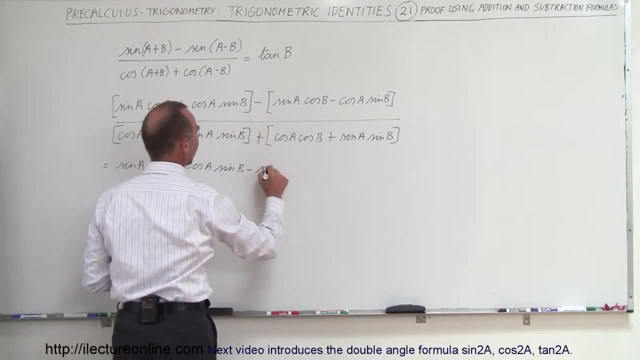 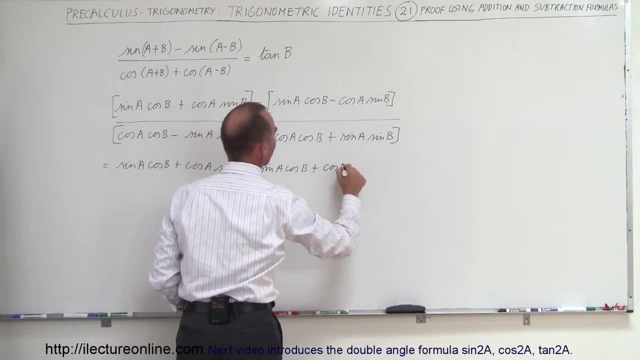 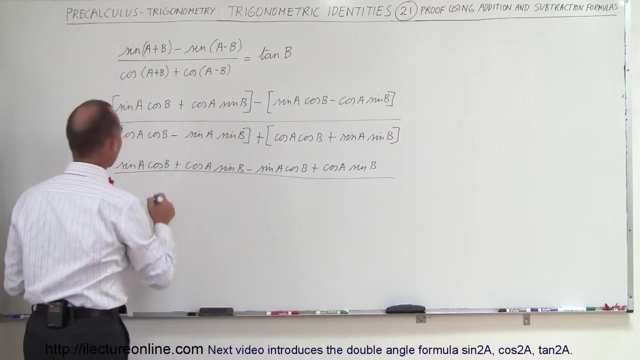 And here we can write: minus the sine of a, cosine of b, and minus times the minus becomes plus cosine of a, sine of b, And the whole thing will now be divided by not quite a straight line, but anyway. so we have cosine of a, cosine b, minus sine a, sine b.